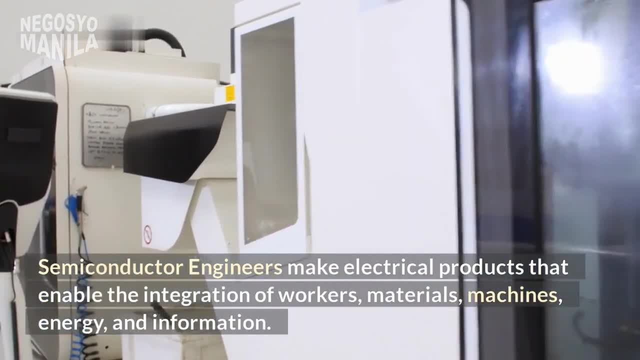 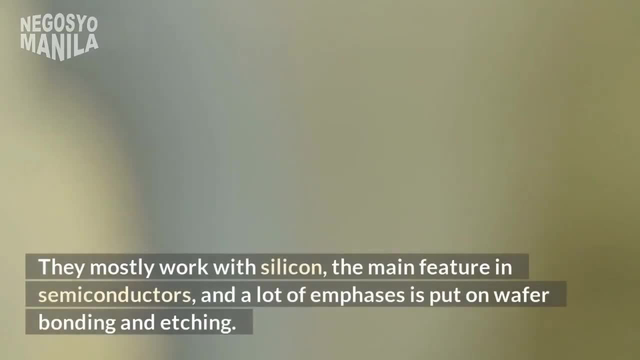 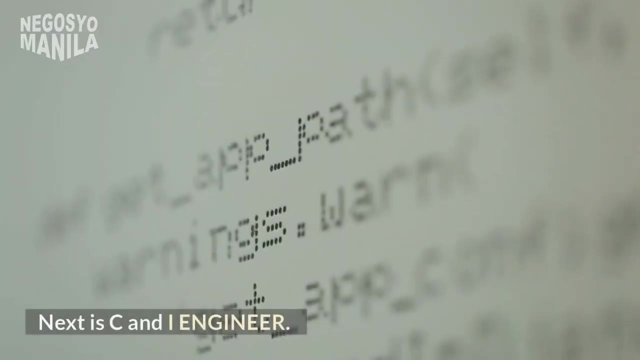 Semiconductor engineers make electrical products that enable the integration of workers, materials, machines, energy and information. They mostly work with silicon, the main feature in semiconductors, and a lot of emphasis is put on wafer bonding and etching. Next is C&I engineer. 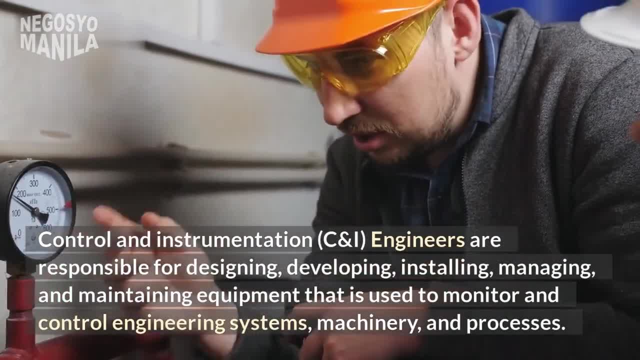 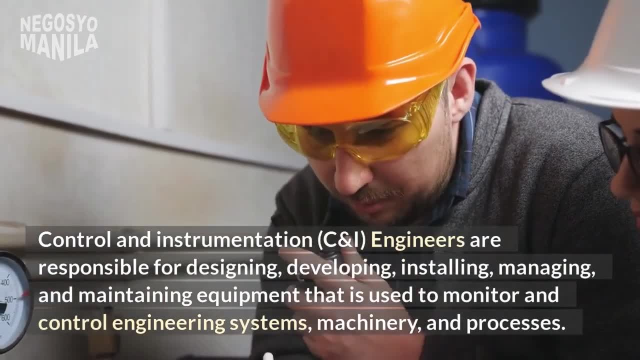 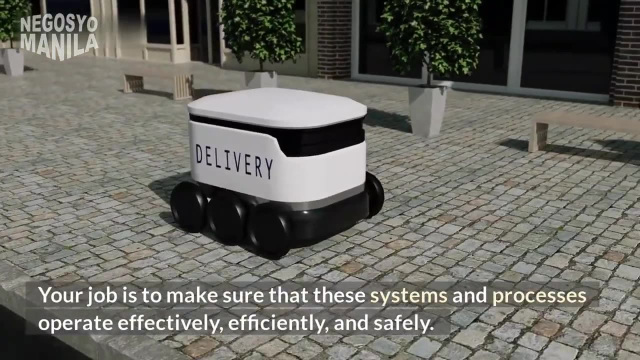 Control and instrumentation. C&I engineers are responsible for designing, developing, installing, managing and maintaining equipment that is used to monitor and control engineering systems, machinery and processes. Your job is to make sure that these systems and processes operate effectively, efficiently and safely. Eight- Power electronics engineer- Power electronics. 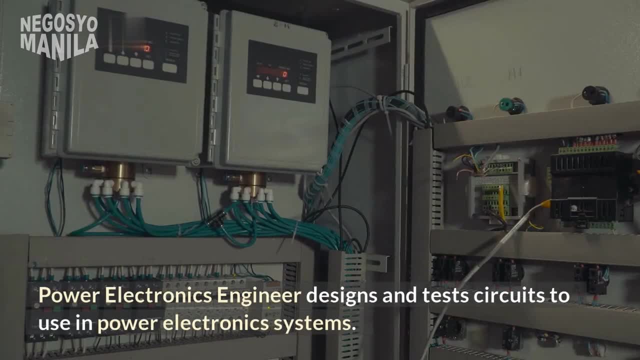 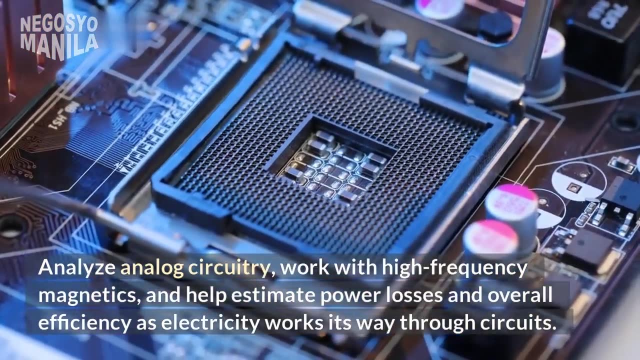 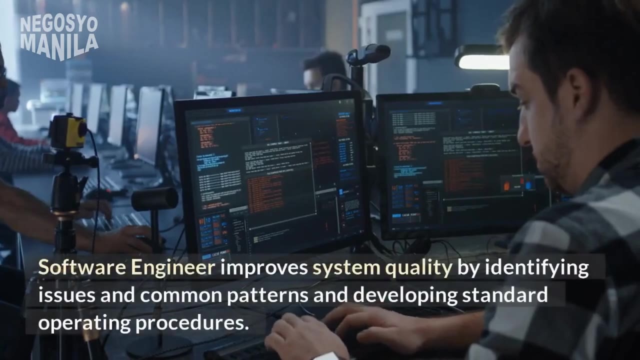 engineer designs and tests circuits to use in power electronic systems, Analyze analog circuitry work with high frequency magnetics and help estimate power losses and overall efficiency as electricity works its way through circuits. Nine: Software engineer: Software engineer improves system quality by identifying issues and common patterns and developing 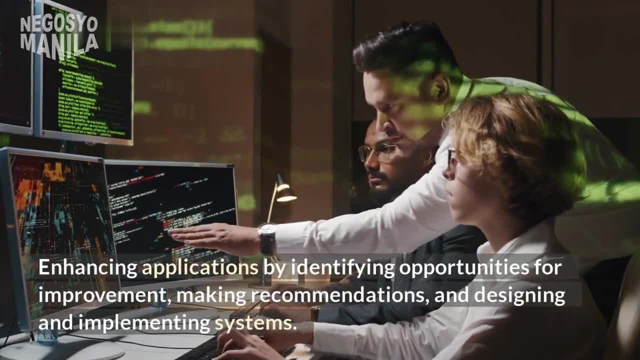 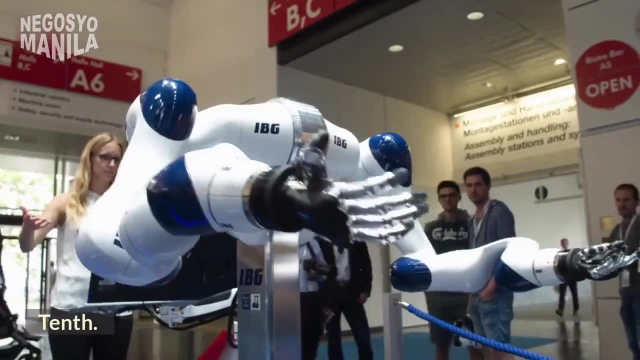 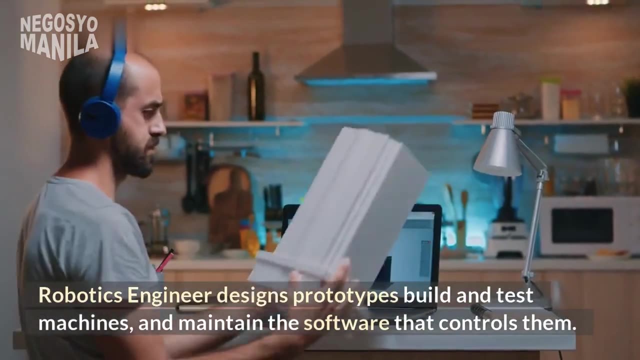 standard operating procedures, Enhancing applications by identifying opportunities for improvement, making recommendations and designing and implementing systems. Ten Robotics engineer. Robotics engineer designs prototypes, build and test machines and maintain the software that controls them. They also research to find the most. 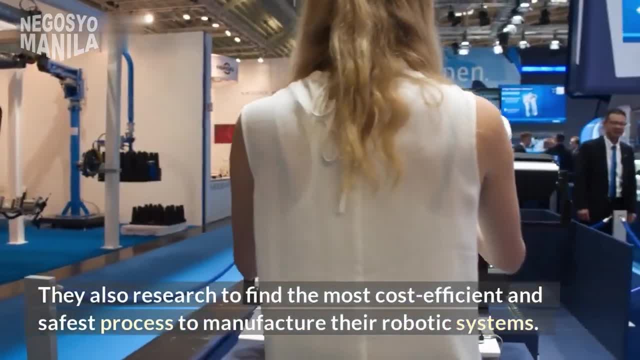 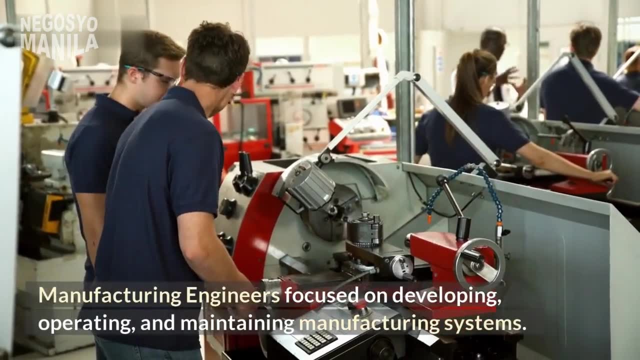 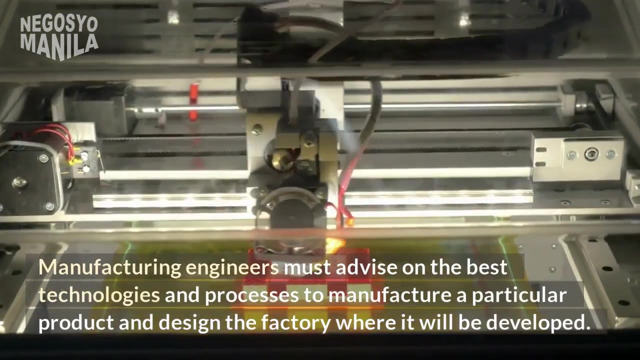 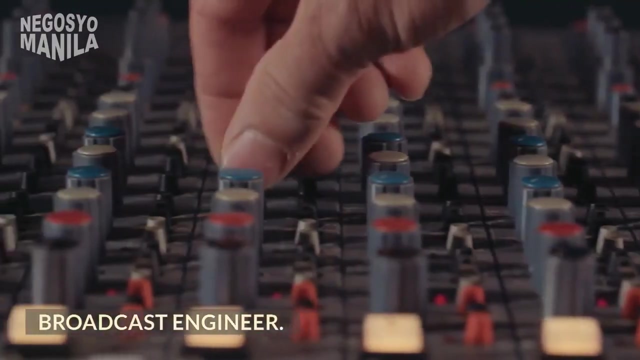 cost-efficient and safest process to manufacture their robotics systems. Eleven: Manufacturing engineer. Manufacturing engineer is focused on developing, operating and maintaining manufacturing systems. Manufacturing engineers must advise on the best technologies and processes to manufacture a particular product and design the factory where it will be developed. Twelve: Broadcast engineer- Broadcast. 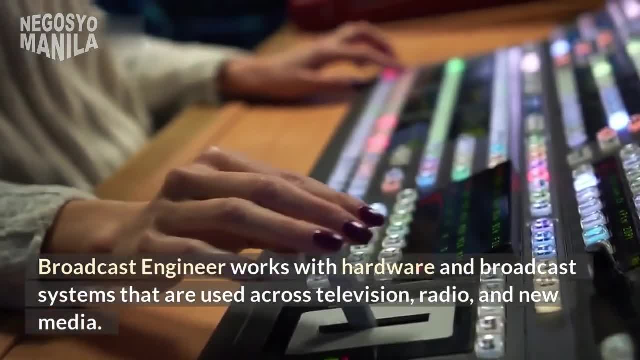 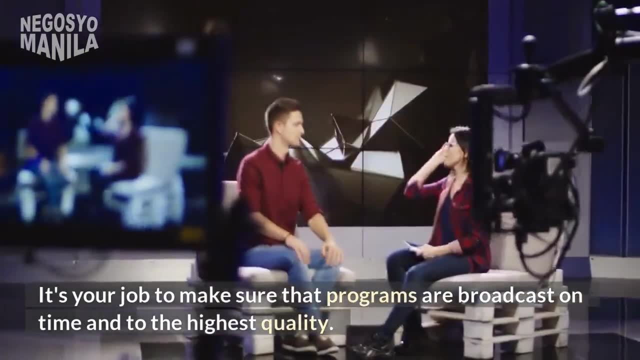 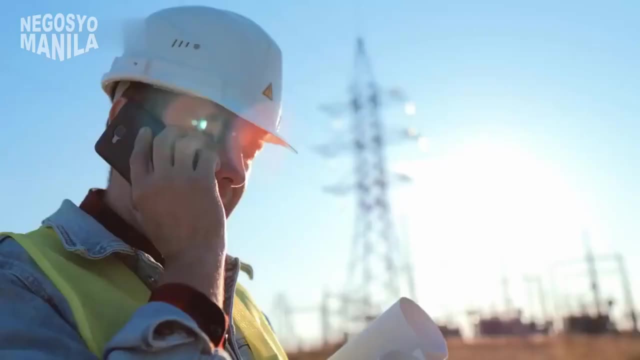 engineer works with hardware and broadcast systems that are used across television, radio and new media. It's your job to make sure that programs are broadcasted on time and to the highest quality. As well as operating and maintaining the systems, you'll carry out updates and repairs. Thirteen Telecommunications engineer. 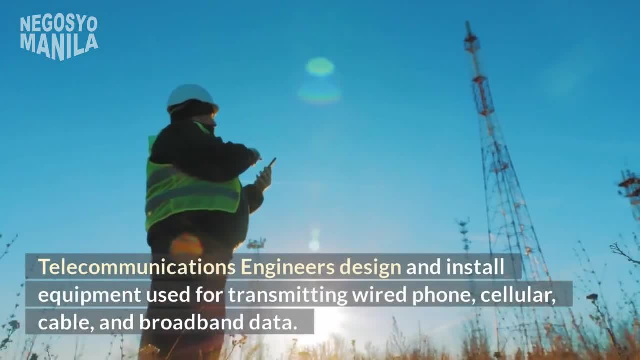 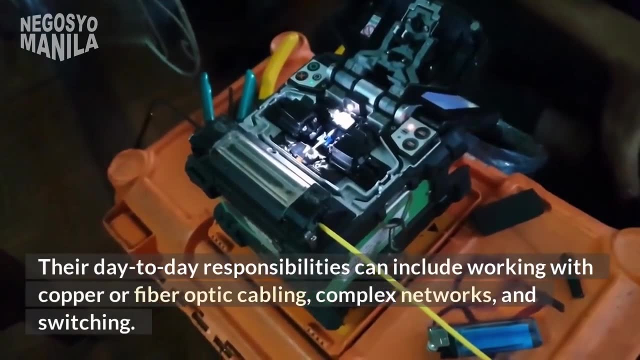 Telecommunications engineers design and install equipment used for transmitting wired phone, cellular cable and broadband data. Their day-to-day responsibilities can include working with copper or fiber optic cabling, complex networks and switching. Fourteen Acoustic engineer. Acoustic engineer works with fiber optic cable, complex networks and switching.